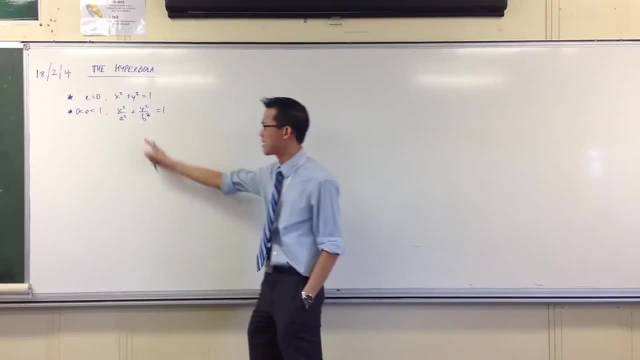 Now, so far, both of them are all centered on the origin. What are a and b? again, What do they control? Yeah, so they control the axes, Right, and they're proportions to each other. okay, And of course, if we wanted to, we could swap them and you get, you know, just taller rather than wider, but oh, all right. 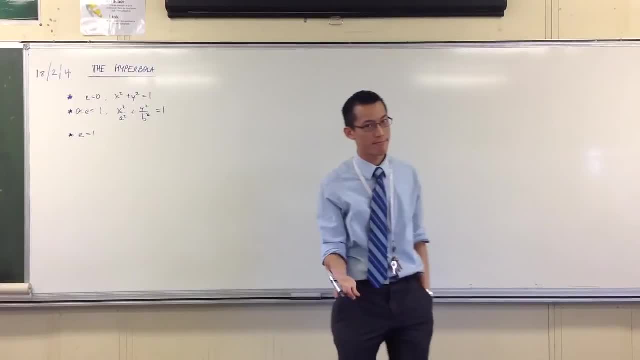 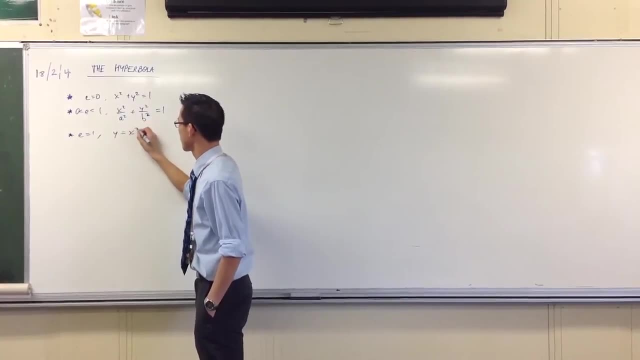 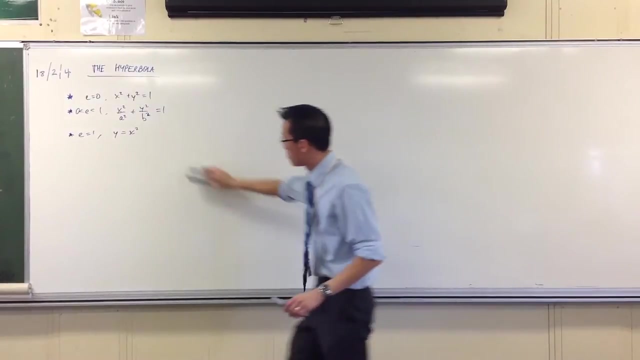 Then you hit this boundary point and you get a parabola. okay, So what's the standard form of a parabola Now, strictly speaking, as we continue up, probably a better comparison would be this guy, Because everything's going to be the same. 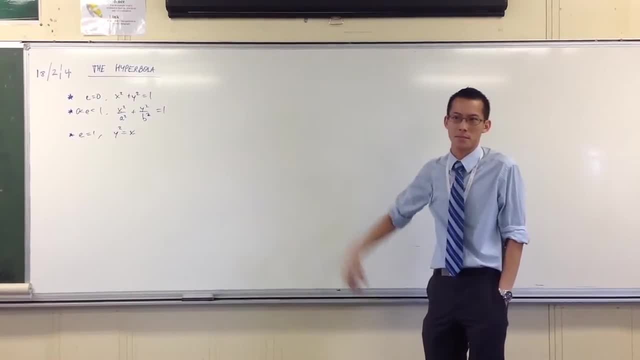 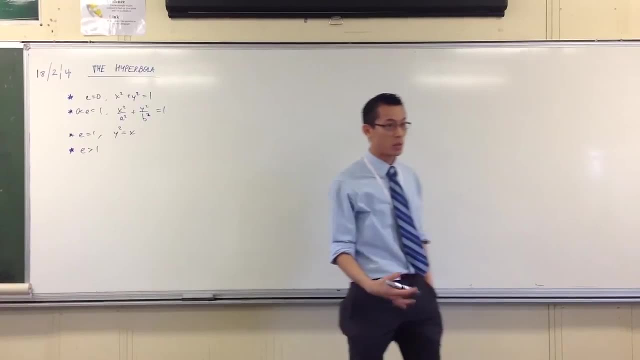 I think we've been looking at it in sideways, yeah, but it's still a parabola, It doesn't matter, okay. Now, our last bit of progress was that we developed this. We looked at it, we tried to draw it and we got this shape out. It's a hyperbola, okay. 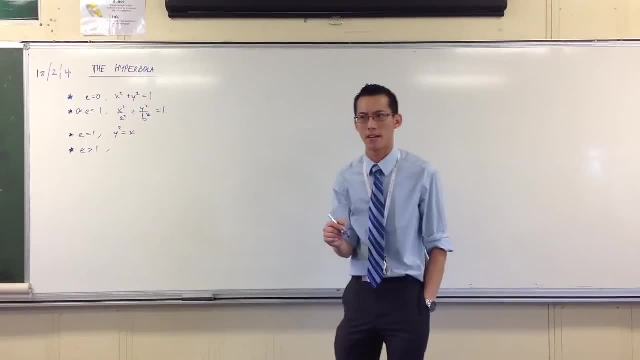 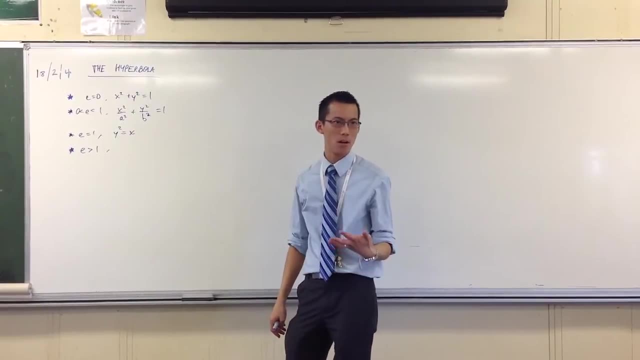 Now I gave you a specific one, right, I think it had, like I don't know, 4 and 12, or some numbers like that. okay, But generally speaking, what's the form of a hyperbola? It's equation. 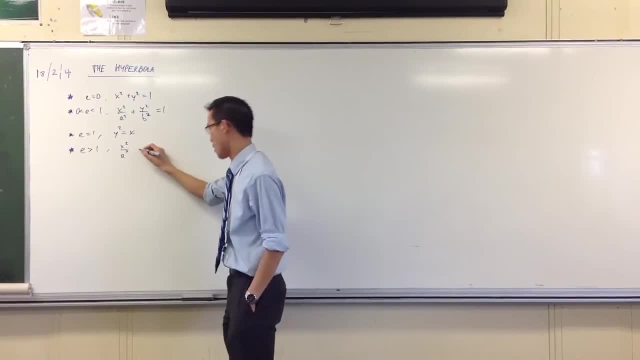 What's the equation? Minus, Minus, Still that, Minus, Minus, Minus. okay, that's what's different? Okay, good, Now you told me very, very, in very detail what these were for an ellipse. okay. 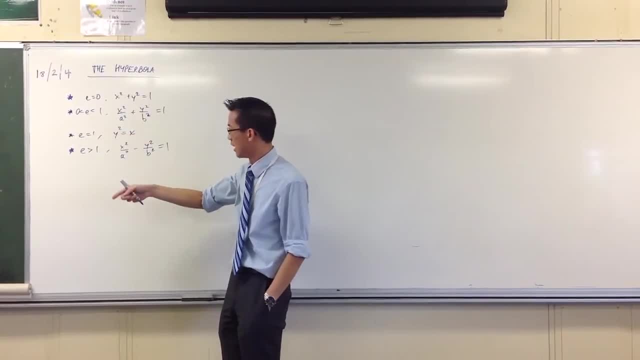 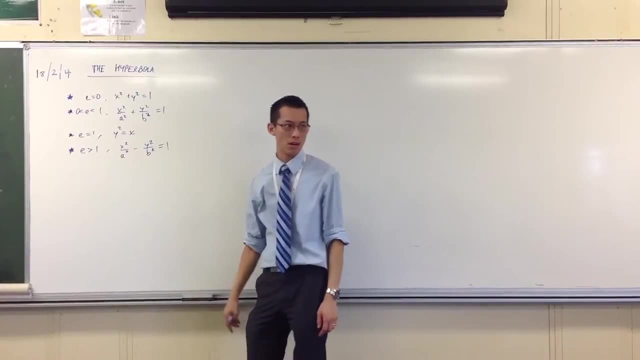 But those features- semi-major axis, semi-minor axis- they don't exist on a hyperbola because it's not a closed shape, right? So my question to you is: what are these things? Obviously there's something important. sort of intuition dictates that it has something to do with the proportions. 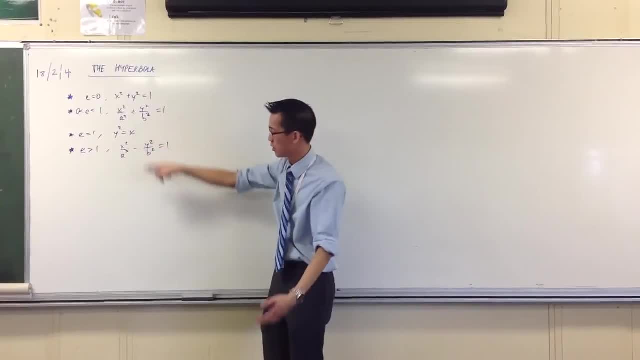 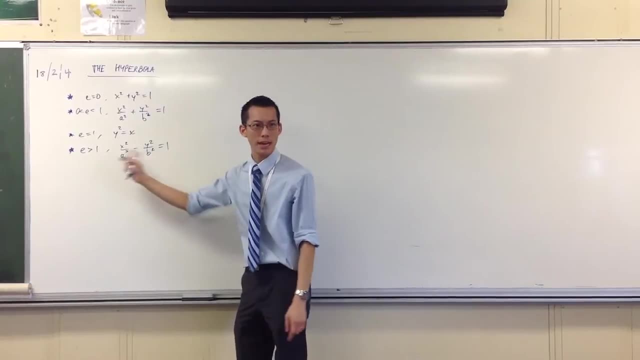 Of the hyperbola, just like this has to do with the proportions of the ellipse. The question is what? Okay, So what I'm going to ask you to do is go back to your drawing of that specific one I gave you. okay. 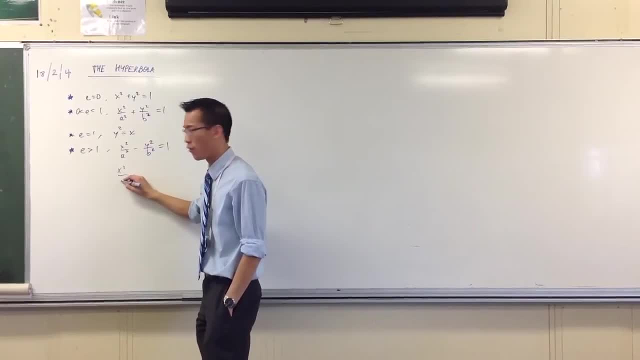 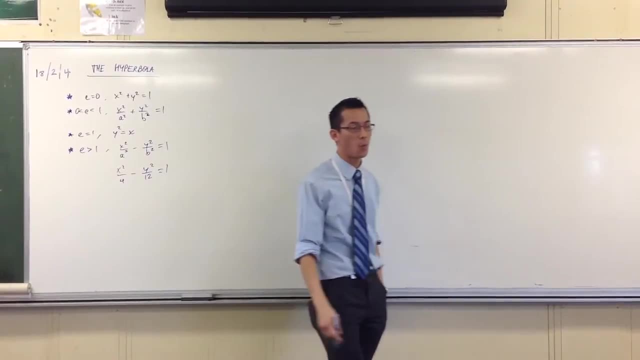 Which I don't know was it. was it 12, or was it 4? 4.. 4, minus, something like that? Yeah, I don't know. okay, Now, what do these numbers signify? Where would they belong? 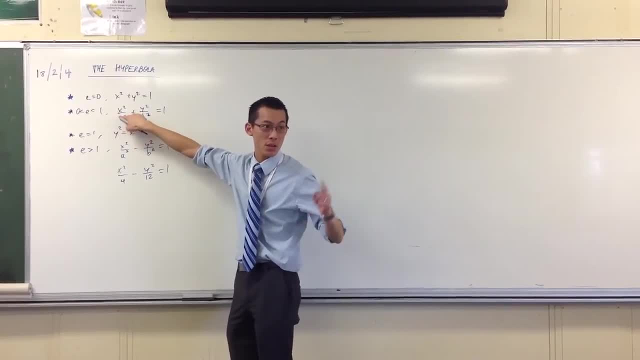 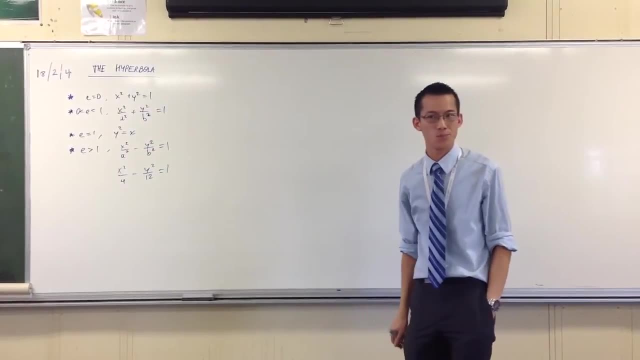 You already know the fact that it's attached to x tells you something. It's attached to x. It's attached to y tells you something. My question is: what exactly is it? What is it referred to? Okay, Now I'm going to ask you to walk through. last time I held your hand through this, okay. 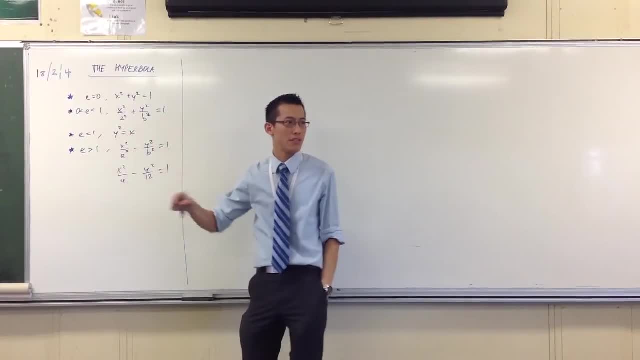 I asked you to get these, and do you remember how we got to that conclusion That they were the semi-major and the semi-minor axes? okay, We generalised this thing and we got this relationship. do you remember this? b squared is equal to. 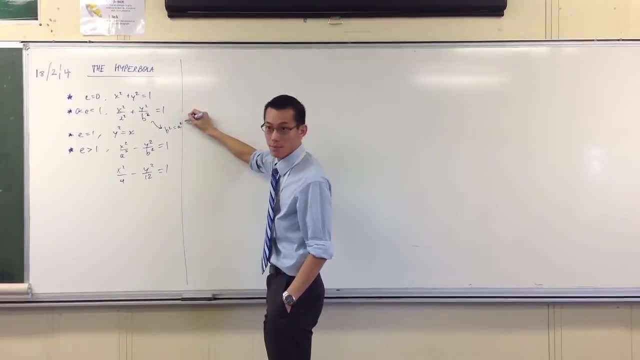 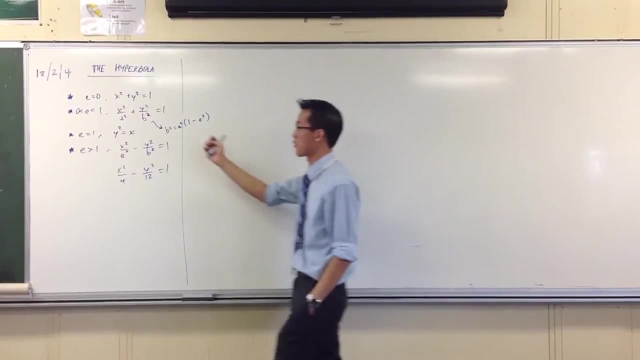 a squared, a squared outside off 1 minus a squared. Okay, we got that right And that's really useful, Because now you can go from an equation and you can get all of the bits and pieces out of it. 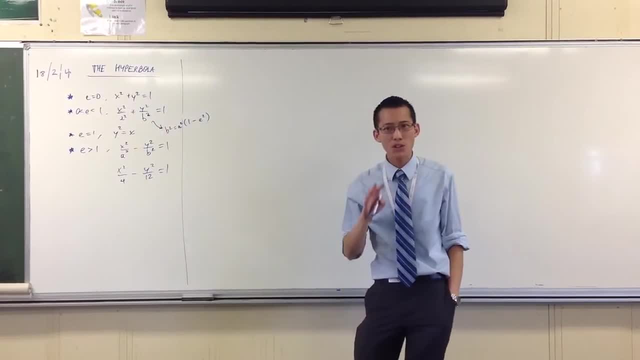 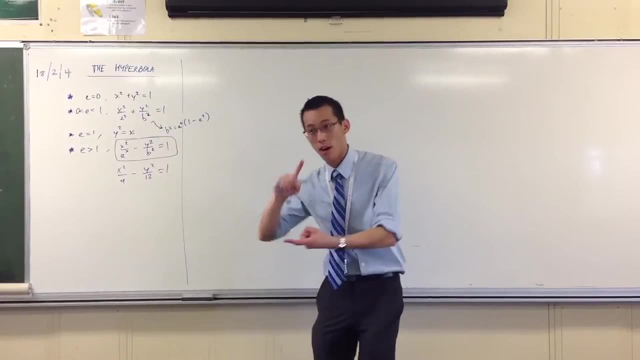 That's really useful. okay, Now I want you to do the same thing, but for this guy. Okay, We started off with a focus and a directrix, and then you got this. Well, if I gave you a different one? 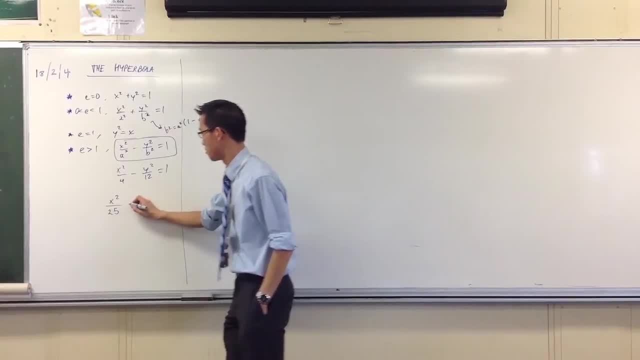 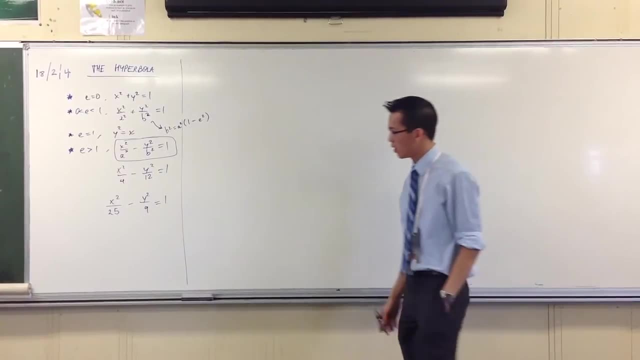 I don't know whatever. 25 minus. I'll give you a nice easy number. Okay, Could you now go ahead and work out where the foci and directrices are and what its eccentricity is? Could you do it? 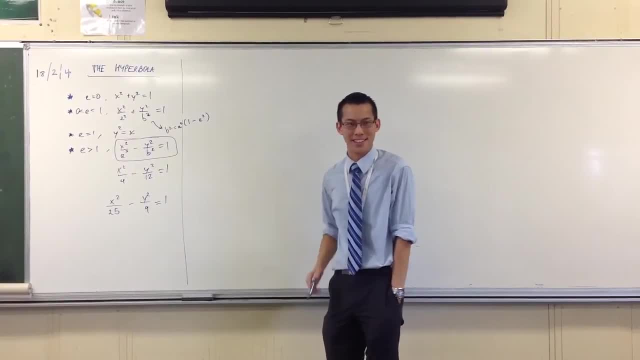 Right Now- probably right now- the answer is no, unless you're really crazy working here. But I want you to try and go back. Think back. if you've got the notes there, think back to what we did with this. 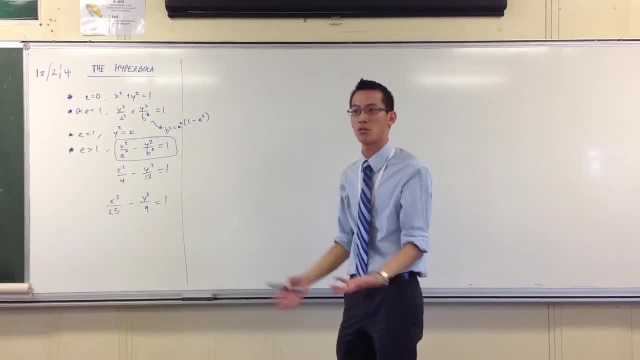 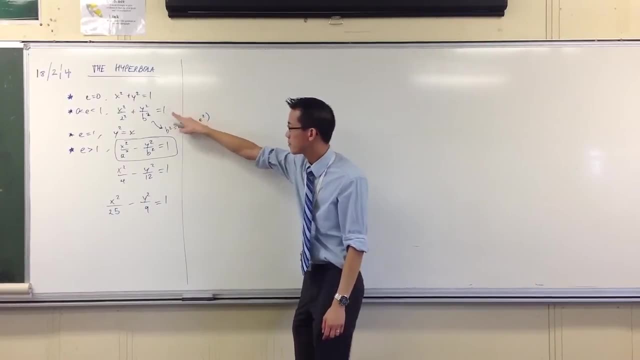 We played some geometric tricks, we drew some stuff, we thought about the general case. We had to look at lines, what they added up to, and so on. Okay, I want you to try and do what you did here here. 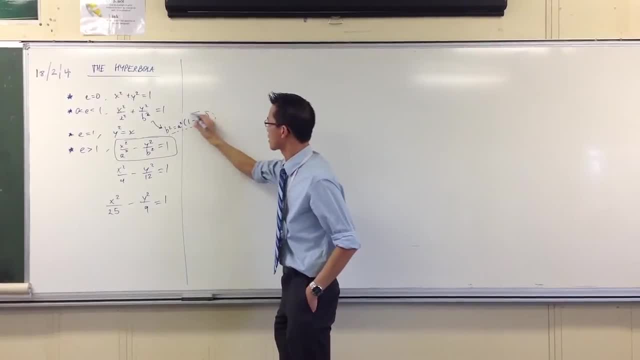 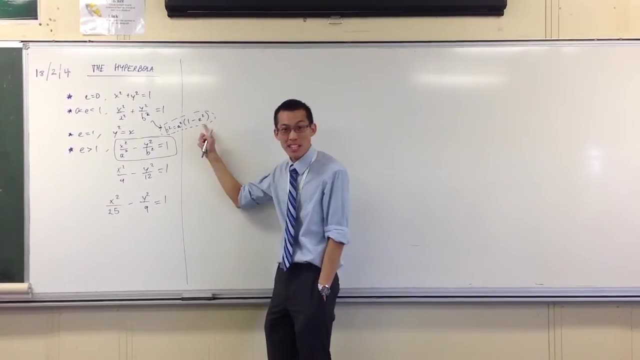 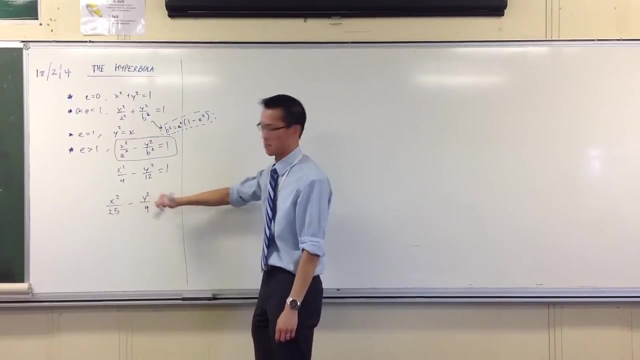 Right, Have a think about this. This guy has a special relationship to the hyperbola, but not in the way that you'd expect. Okay, I want you to see what relationship this has to this. And then our final, where we're trying to head to here, is if you were to get an equation, a hyperbola, right? 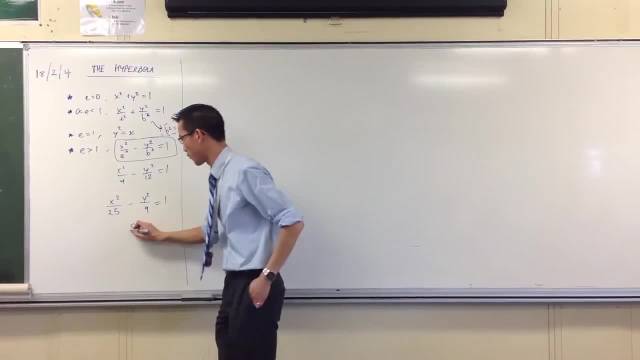 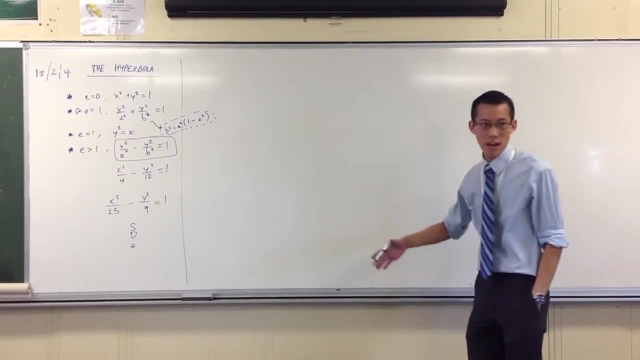 Can you give me all of its features out of it? Can you tell me where the focus is, What the directrices are, What the eccentricity is? Okay, So I'll walk through that with you shortly, but I'll give you guys a five or ten minute head start. 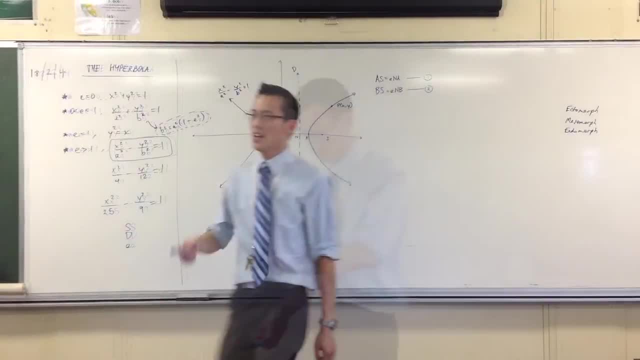 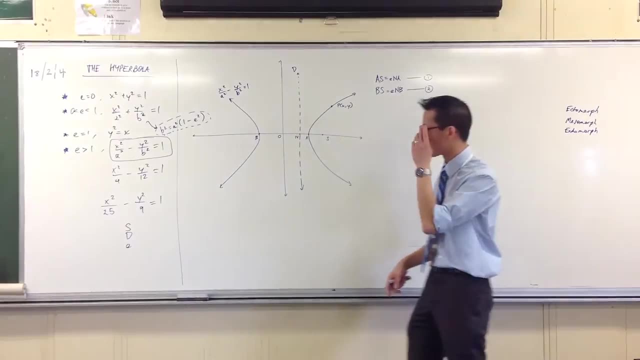 Okay, Off you go. So I'm interested that so many of you, or so few of you, are. let's stack your hands up to see how much progress you are making, Because the way you go about this and the results you get from it are almost identical. 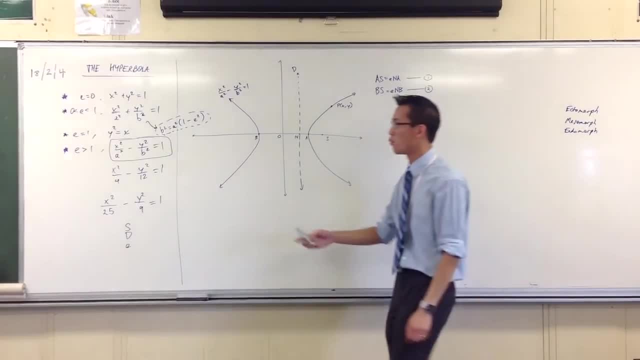 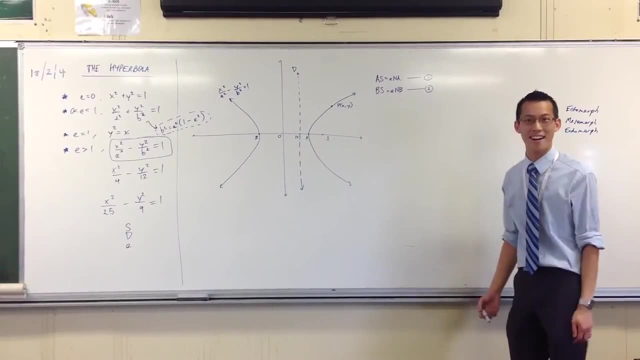 Like down to the The letter from what we did with the ellipse. Okay, So, as If results start seeming familiar, that's because they are Alright. So here's my diagram Right Now. you'll notice what have I done here. 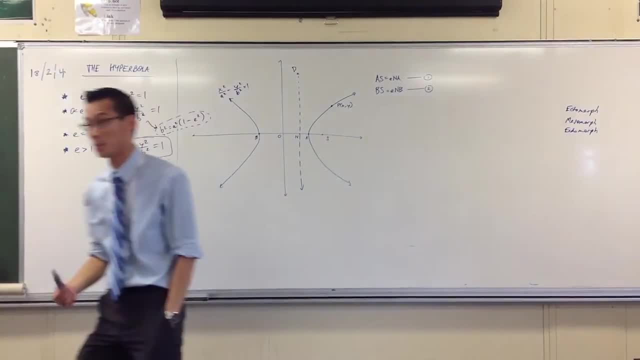 I've set up almost exactly the same two equations I've set up with the ellipse Right, Do you remember them? This is about the definition, like the locus definition, of what the hyperbola is. Okay, So you've got this ratio. 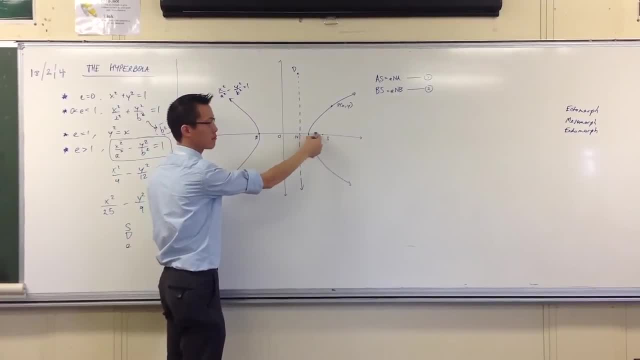 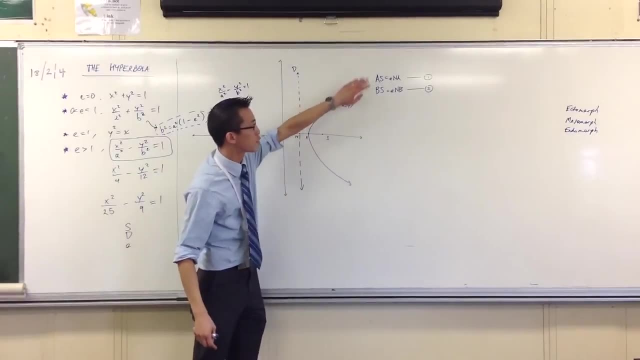 Sorry. Distance of the From your point To the focus Versus the distance to the directrix, And that ratio is E, Right. So I've picked that out just for two points, A and B. And there are my ratios. 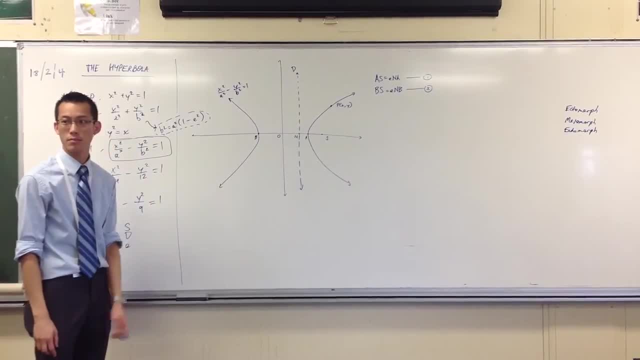 Okay Now, do you remember what we did with those equations last time? We did two things: Firstly, we added them and then we subtracted them, And then we saw cool, useful stuff out of them from that. Okay, So let's give it a go. 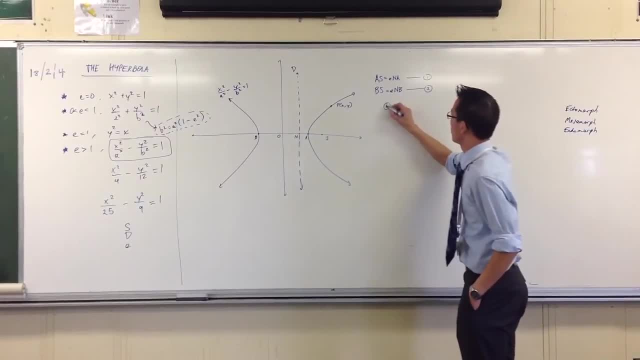 What happens if we add them? Let's do adding first. Okay, What do you get on the left-hand side? A, S Plus B. That's convenient. A plus E And B- Okay. Now the question for you is: how do we combine these into something meaningful? 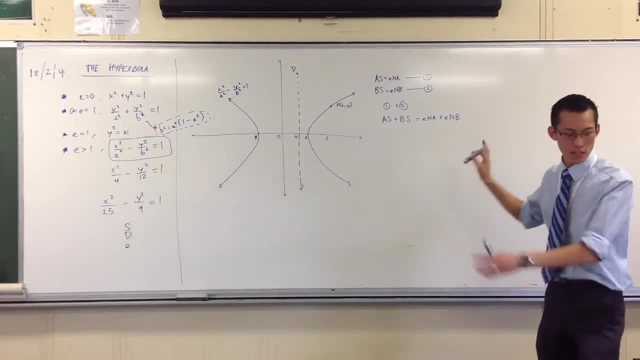 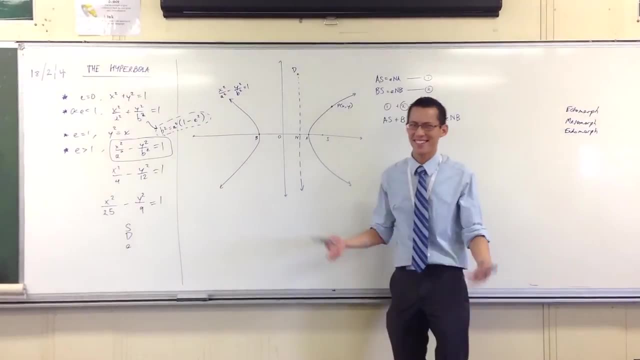 Okay, Now B S Plus A S. Okay, It's not my fault. Okay, You can read the textbook. That's what they pick out. Okay, What distance is R X Plus A X Plus A X? 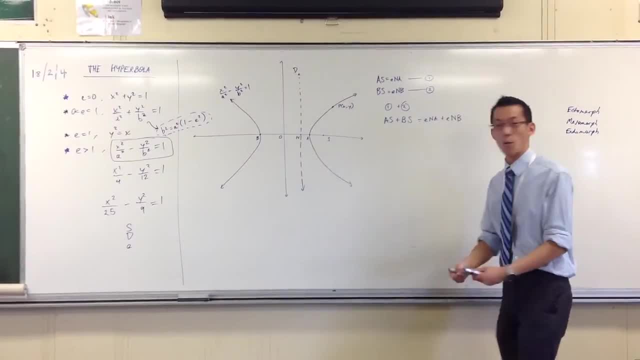 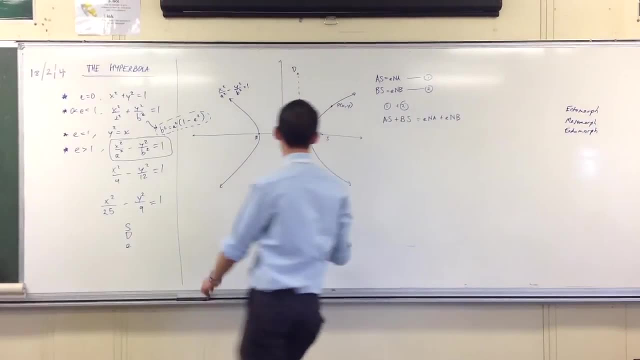 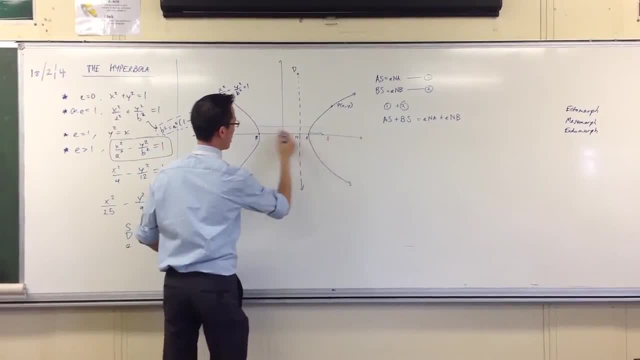 Okay, Now don't forget where am I trying to head to. in case you couldn't remember, I'm trying to get the focus. I'm going to try and get the directions. The eccentricity comes quite a bit later here, Remember. 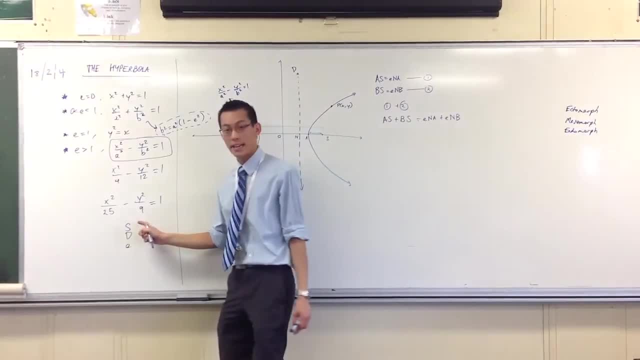 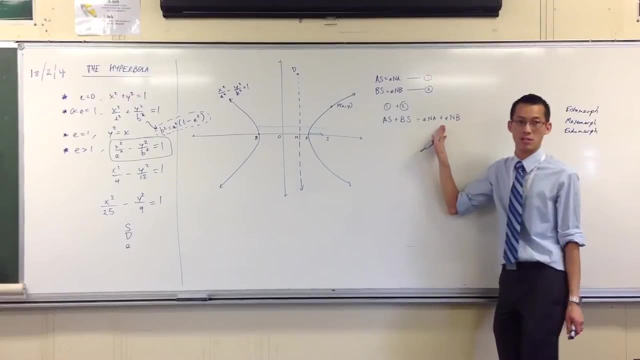 Okay, Because we're working in terms of eccentricity, so we shouldn't expect to be able to get something what it's equal to, Right? So these two lengths, they're going to be equal to a distance of, say, a meter. 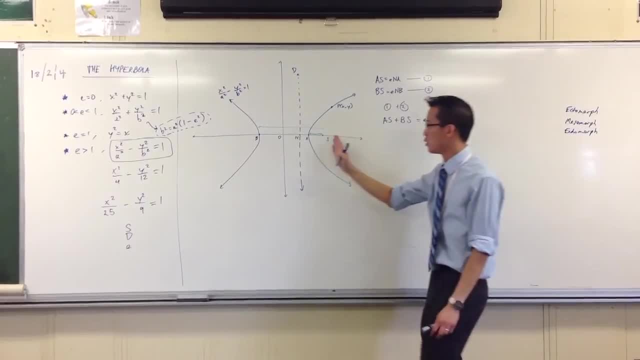 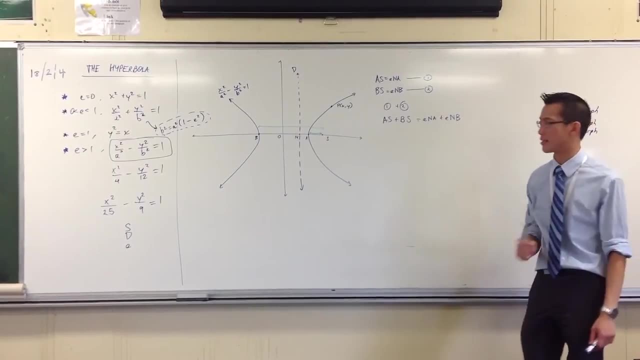 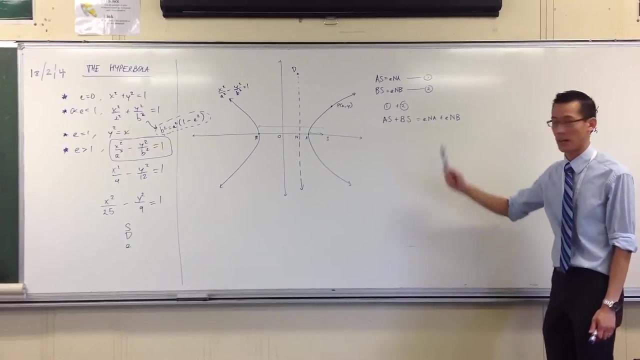 Right. So what are we going to do? lens: have a look. what do they relate to most right? well, because they're both defined by s. they should tell us something about the distance to the focus, shouldn't they? that's nothing to do with the directrix, which is n okay, so 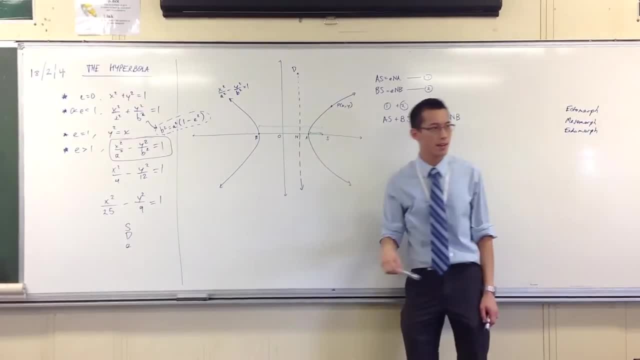 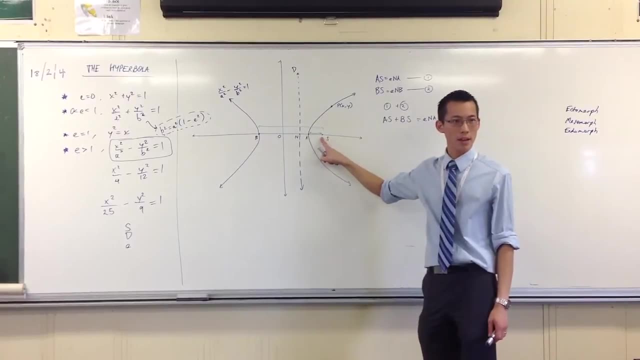 therefore, when you add these two green links together, they should give us something close to something that's related to the focus. right, the focus is here. okay. now if I were to find out the coordinates of the focus for this particular diagram, okay, what would its coordinates be? let's do these one what's. 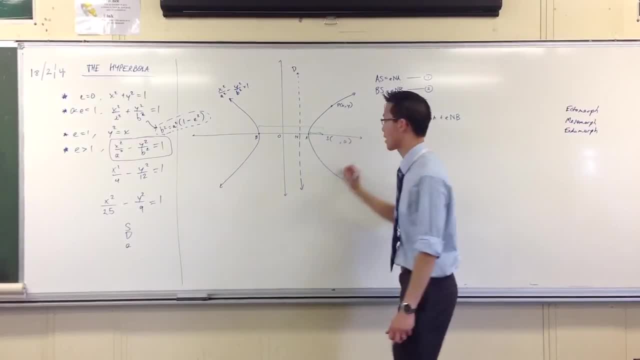 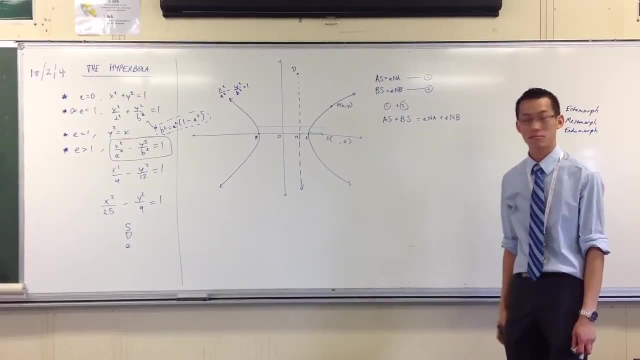 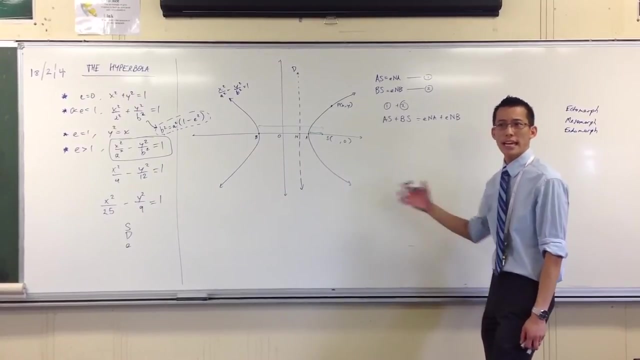 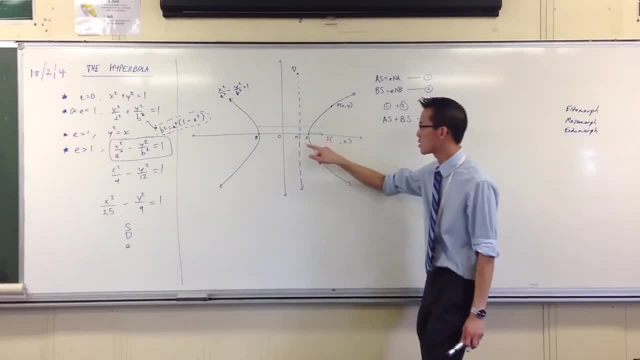 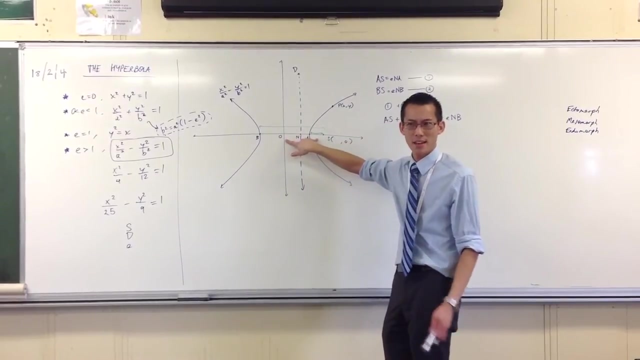 I have here now looks to me like you know, suppose this, this coordinate was five, suppose. okay, tell me, what would this distance be? five, wouldn't it? if this was three, what would this distance be? so the coordinate comes from this distance. see that, because the distance from the origin, right. so you could say: 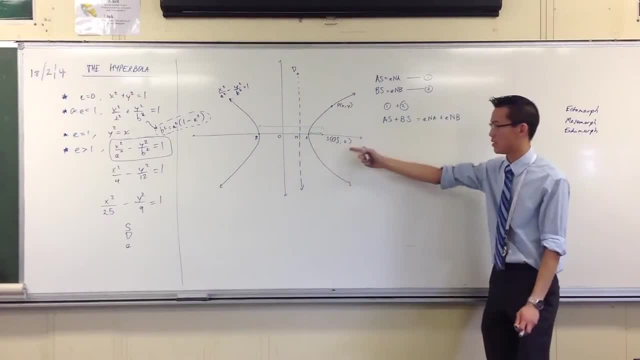 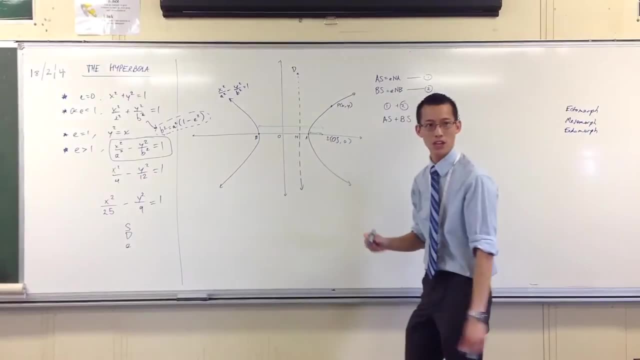 it's OS, whatever, that is zero. okay, now, these two links are related to OS, that distance there. can you see it? how are we going to chop and change? to make it obvious, what would you chop up? you can move around the short distance or you can chop up the longer distance and 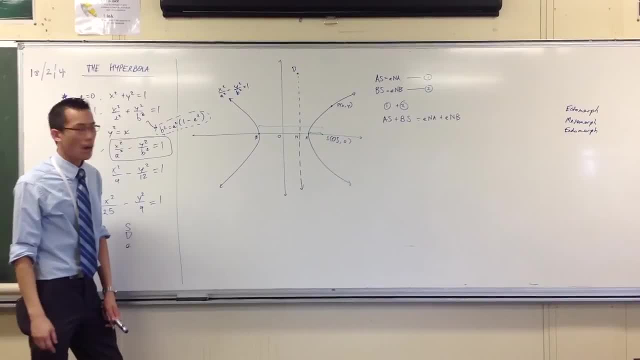 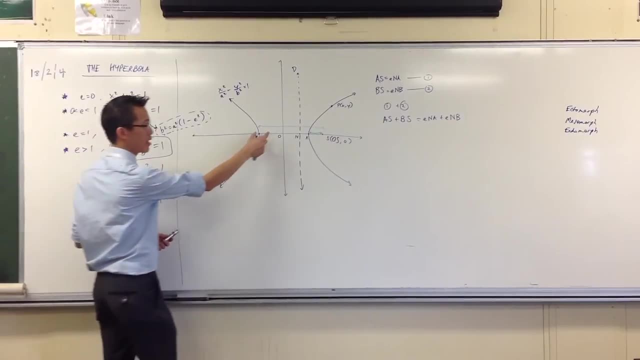 rearrange that. I'm thinking you think back to your lips how we did it. personally, I would take OB. look at OB, see that distance there. yeah, distance. I'm thinking. think back to your lips how we did it. personally, I would take OB. look at OB, see that distance there. see that distance. 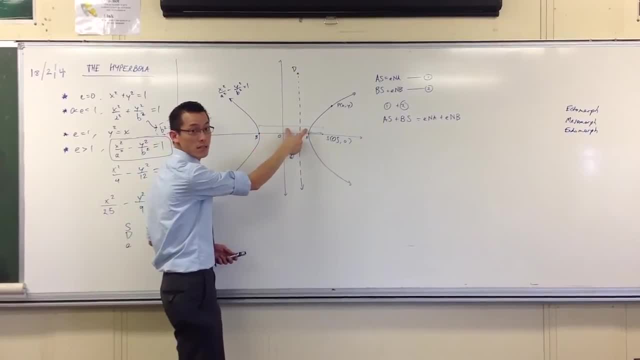 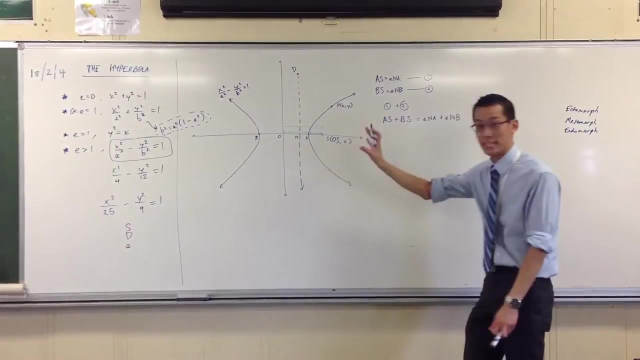 what's the relationship between the OB distance and the OA distance? it's the same. so this symmetry here, right, so I can move this guy over here. now, when I add them up, what is AS bs? it's double that distance, right, two times the distance of the focus from the origin. 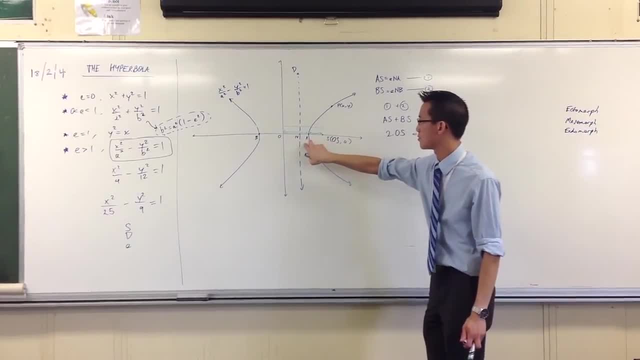 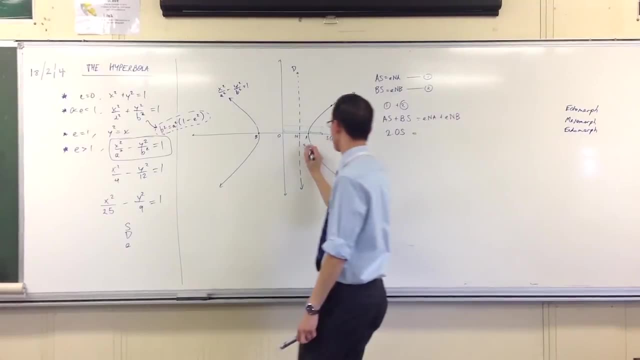 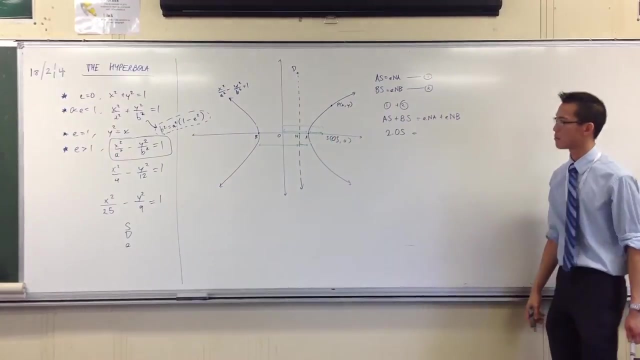 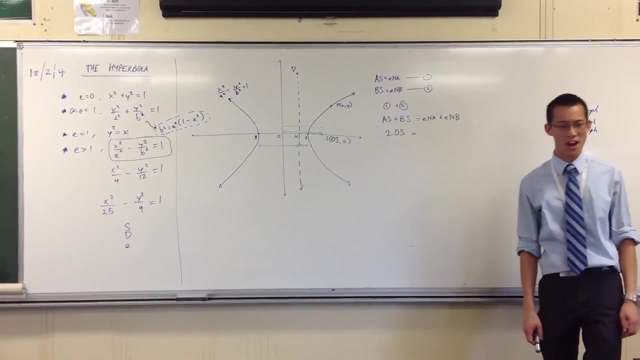 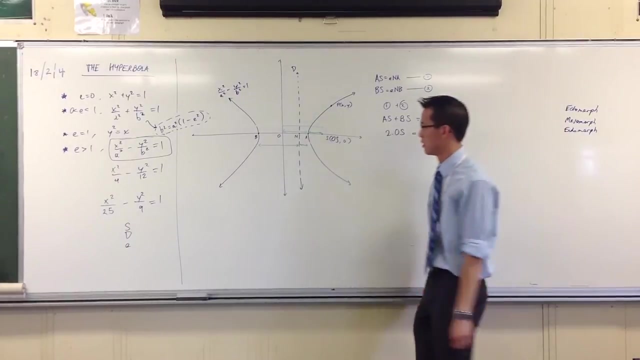 what about this? MA MB? Can you see it? I'm running out of bubbles In A and in B. Come on, I helped you out with the first one, Can you see it? It's going to be well. it's just that whole distance, right. 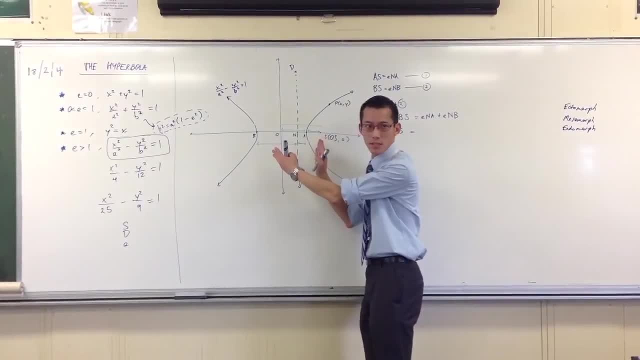 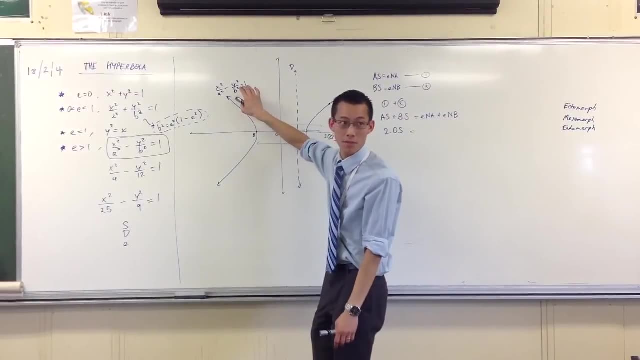 But hold on a second. We know what this distance is, don't we? Because I've called this capital A. but I actually know where it is Because I have the equation of the hyperbola right. What are the coordinates of capital A? 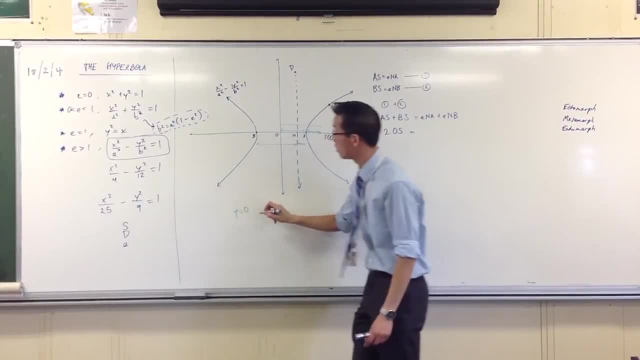 You'd say: well, it's on the axis. so you say y equals 0.. So that means x squared on a squared minus 0 is equal to 1.. So you've got x being plus or minus a. So here's 1.. That's plus a. 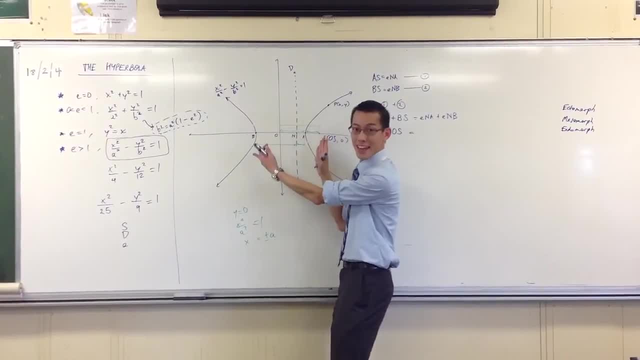 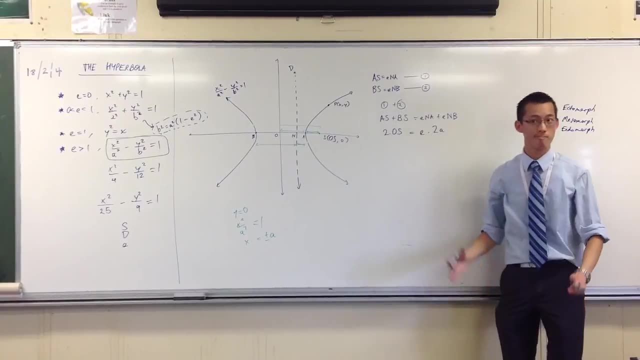 Minus a. So what's the difference between plus a and minus a? It's 2a, isn't it? There's an e there Times 2a. Okay, So 2s cancel. So OS is equal to. 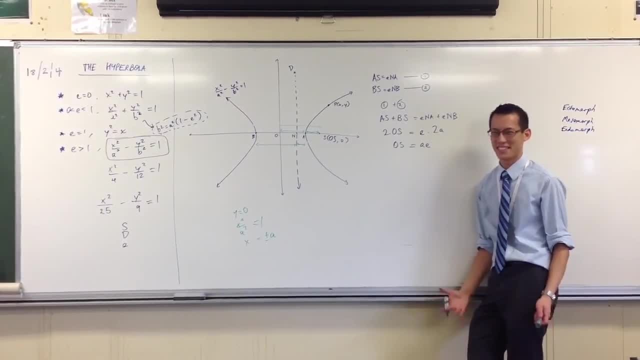 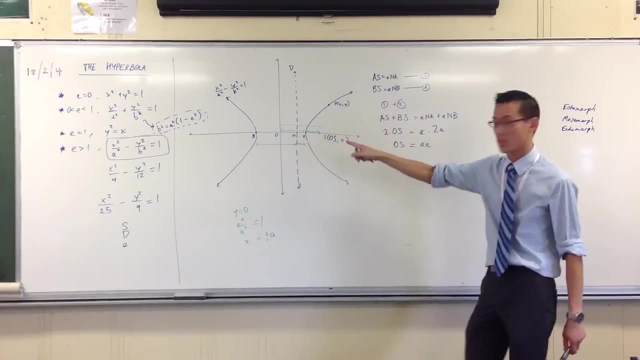 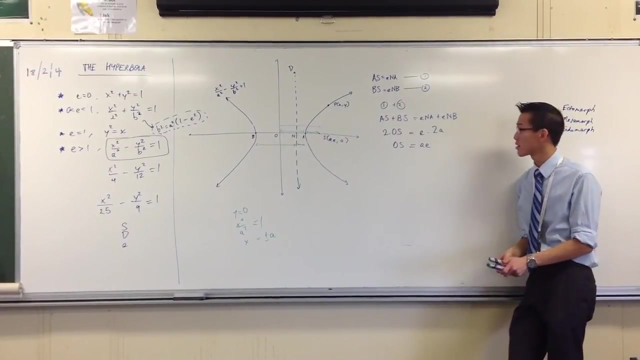 oh, that's familiar, isn't it? Tell me that's familiar. Okay, That's that distance there. So if I can now fill that in, that tells me the coordinates of the focus are a e, 0. Which shouldn't surprise us. 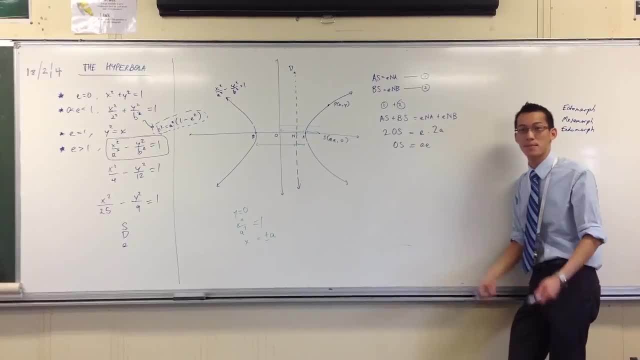 because all of these equations are exactly the same as the ones we did for the ellipse, Like line before line. they're exactly the same. So therefore, let me do a bit of a shortcut If I'm trying to work out where the directrices are going to be. 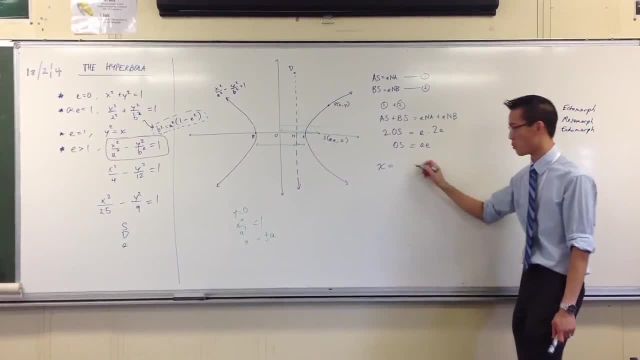 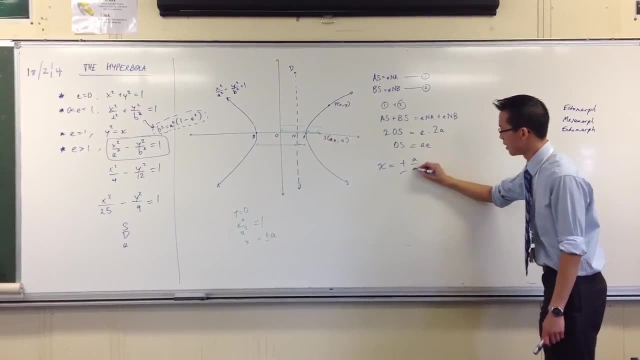 they would be in the form of an equation: x equals plus or minus something. Could you make an educated guess? What's the equation of the directrices A or A?